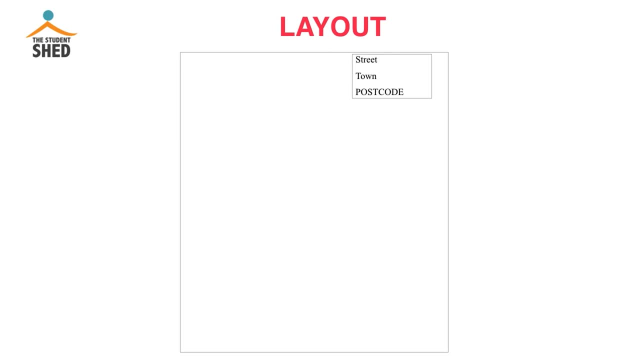 see in front of you and on the right hand side, you would write your own address there and beneath that you would include today's date. So your address on the right with today's date beneath. Now, on the left, you would include the name of the recipient. It's important. 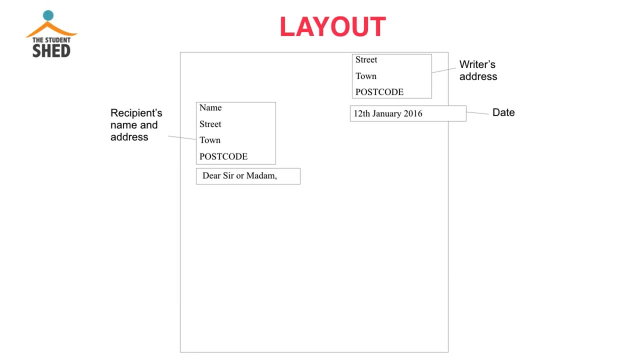 to do that for a formal letter, and then, beneath that, you start off with a salutation: dear sir or madam, or if you know the name of the person, you could include their surname: dear Mr Thompson, etc. Now, once you've done that, you could start your letter with highlighting: 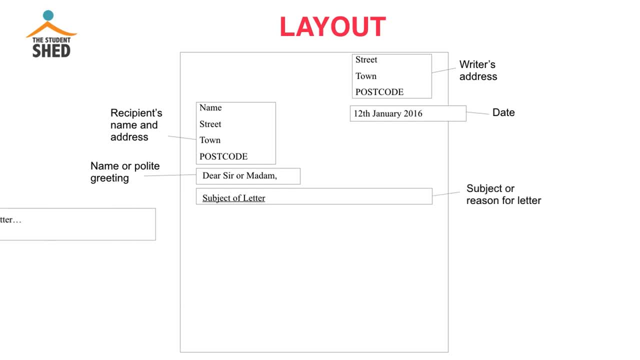 the subject of the particular letter that you're writing, and then, beneath that, you need to include the main point of the letter, So you can start off by talking about what the letter is about, and this may extend into more than one paragraph. When you've finished writing your letter, you would then conclude: 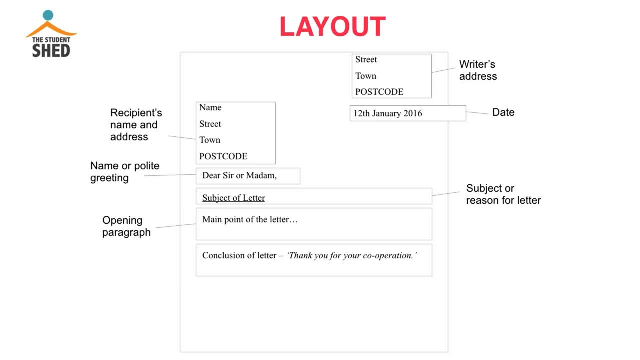 often by saying thank you for your cooperation or similar, and then at the end of the letter you need to finish with the sign off: yours faithfully or yours sincerely. We'll talk more about that in a moment, about when to know, when to choose faithfully or sincerely. 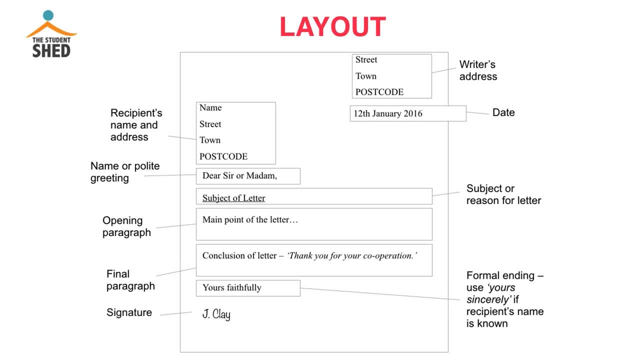 You would then sign your name and just for clarity's sake you would then have a little mistake. You would print your name at the bottom of the letter so that the recipient definitely can identify who you are. So that's the layout for a formal letter, and all formal. 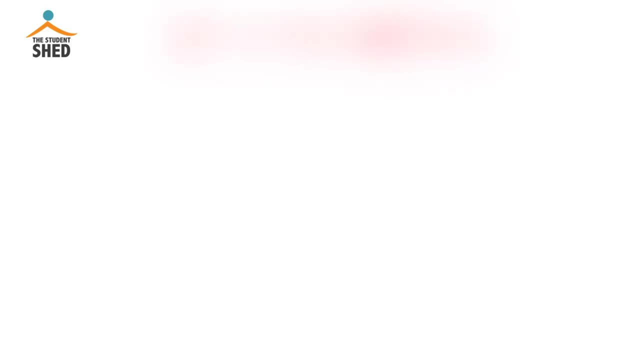 letters should follow that format. Okay, moving on then to look a little bit at structure and tone of formal letter writing. The first paragraph, as we said, should be explaining why you are writing to the recipient. You need to explain who you are so it's clear to them, and you need to be polite If you 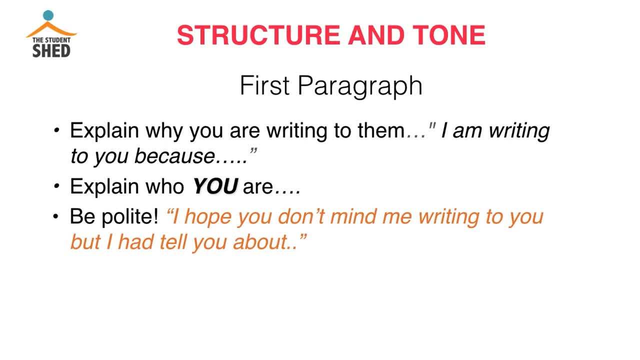 are writing to the recipient. it's important in terms of tone for a formal letter to be polite at all times, even if you are complaining, It's also important to be strong. so if it is a letter of complaint, you need to make sure that you are quite forceful in putting. 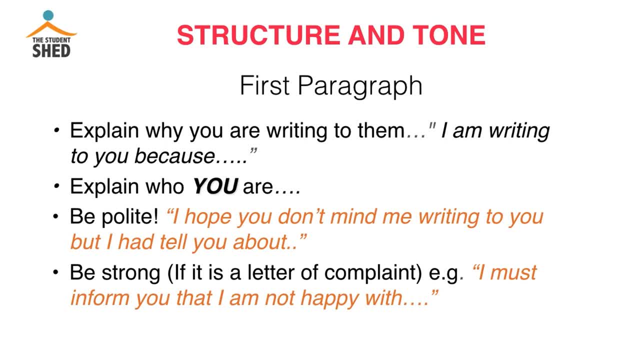 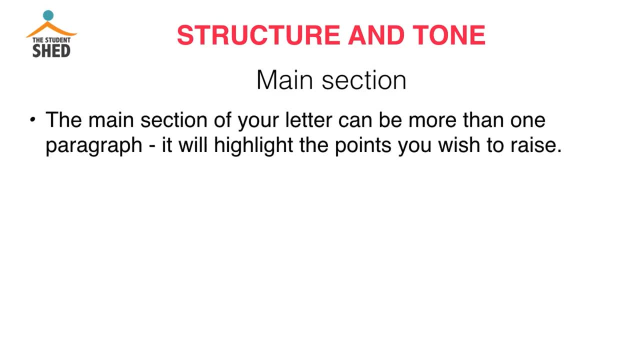 across your point of view. So be polite, but also be strong when writing a formal letter. So, moving on to look at the main section of your letter, As we mentioned previously, it can be more than one paragraph, but it's going to highlight the main points that you wish. 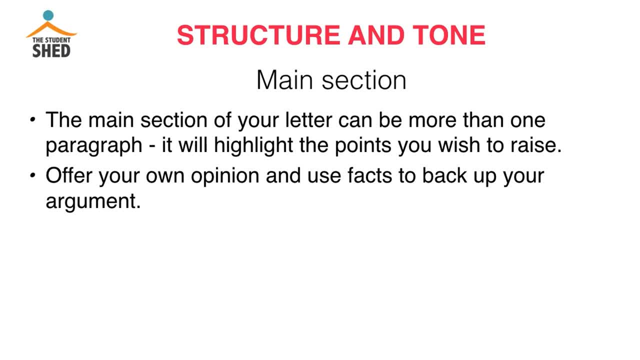 to raise. It's important here that your own view is reflected. so offer your own opinion here, and if you have any facts to back up your argument, then of course do use those in this section of the letter. It's important for your letter to be coherent, so make sure. 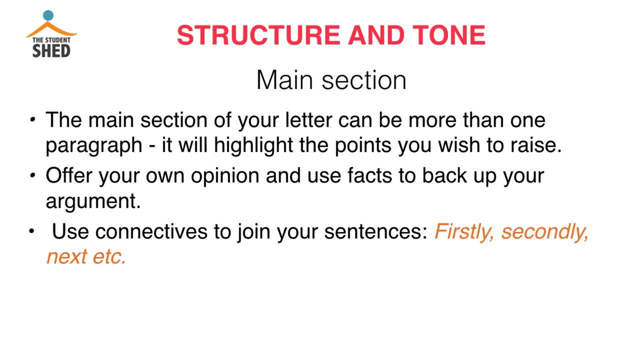 you use connectives such as firstly, secondly, to structure the letter and make it clear for the reader what you are trying to say. So, overall, it's also very important to make sure that you check your spelling, as formal letters would be expected to have. 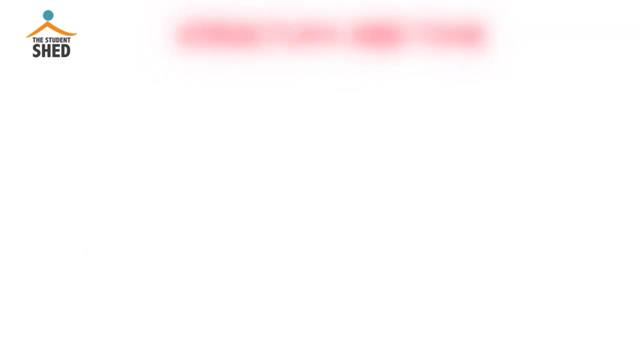 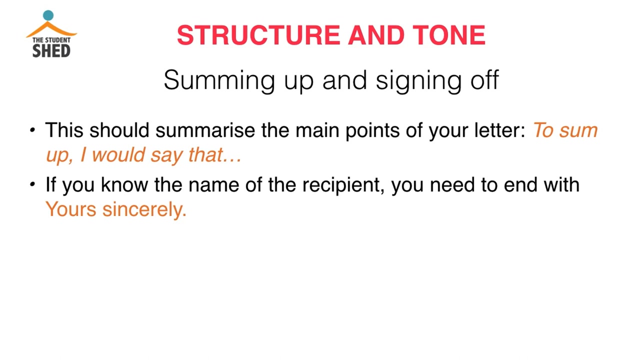 perfect spelling throughout. Ok, we mentioned before that you need to sign off at the end of the letter. Before that, you would just sum up the main points in the final paragraph and then, if you know the name of the recipient, you would use the ending yours, sincerely. So, for example, if you used: 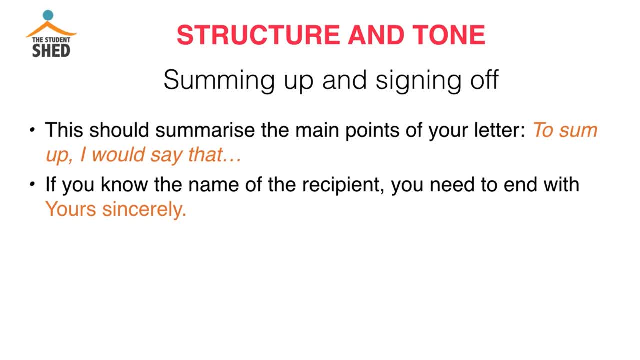 yours. sorry, if you used dear Mr Thompson, you would end that with yours sincerely. If you don't know the name of the recipient and therefore you've started the letter with the words dear sir or madam, you need to end with yours faithfully. Now there's quite an easy. 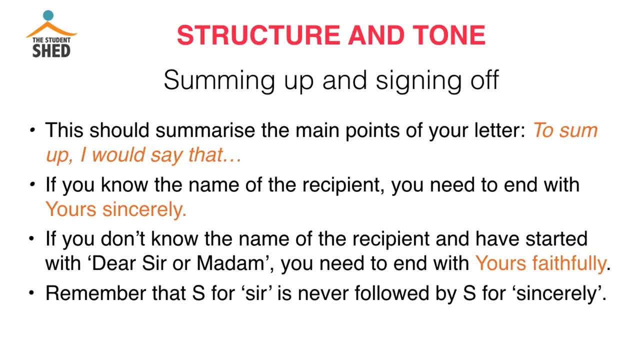 way to remember this. S obviously is the initial letter of the word sir, and it's also the initial letter of the word sincerely. Well, these two would never appear together. So if you put dear sir, you would never put dear sincerely. you would put yours faithfully. So if you 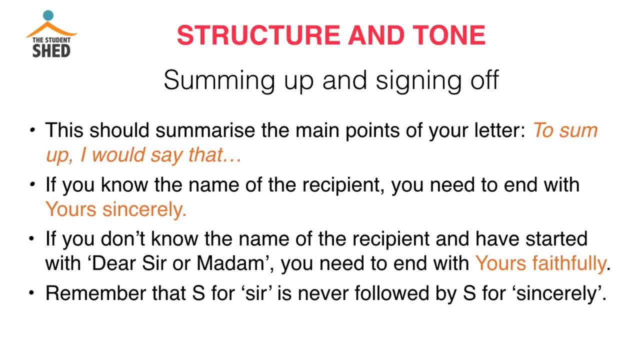 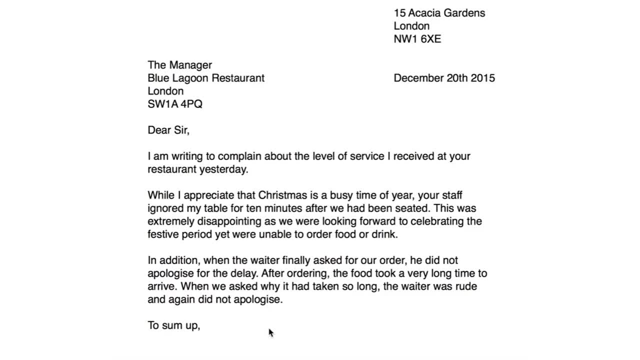 see two S's together. you've got it wrong. If it's dear, Mr Thompson, it would be sincerely, and if it's dear, sir, it would be faithfully. So an easy way to remember which to choose at the end of a formal letter. So here's an example of a formal letter. This one is from 15 Acacia Gardens in London. 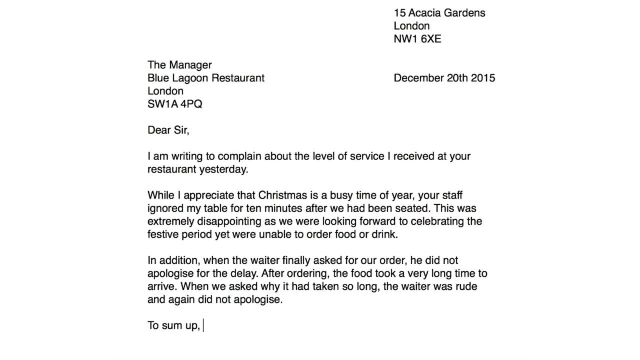 to the manager of the Blue Lagoon restaurant. It begins: dear sir, because they don't know the name of the manager. and then it says: I'm writing to complain about the level of service I received at your restaurant yesterday. A very clear opening sentence there. Then the 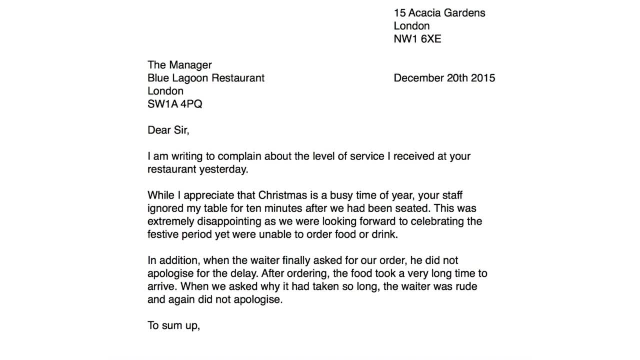 main body of the text can be seen there, talking about Christmas being a busy time of year, but staff ignored the table for ten minutes when they'd been seated and that was extremely disappointing. They also point out that the food took a long time to arrive and there 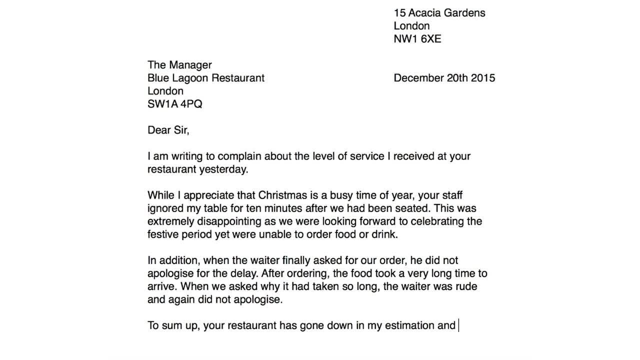 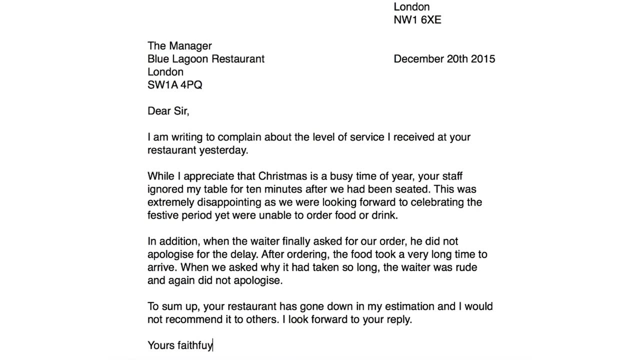 was no apology for that. So if you look down to the bottom now where the letter is being completed, To sum up, your restaurant has gone down in my estimation and I would not recommend it to others. I look forward to your reply. OK, so suggesting that this person wants a reply from the restaurant, Now it's yours. 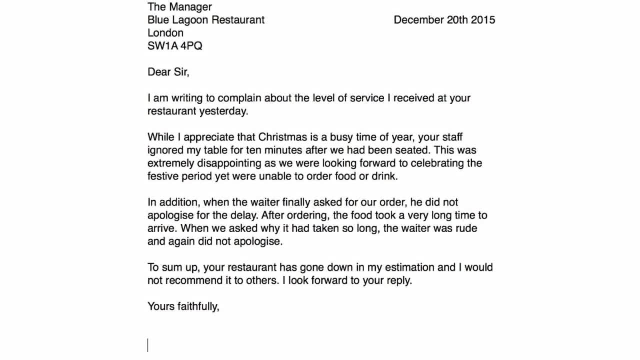 faithfully, because it's dear, sir. so you would never have two S's together And here the name John Smith. If it had been printed out, obviously the signature would go just above John Smith and below yours, faithfully. So there you go. if you wanted to freeze the screen and have a read of that, 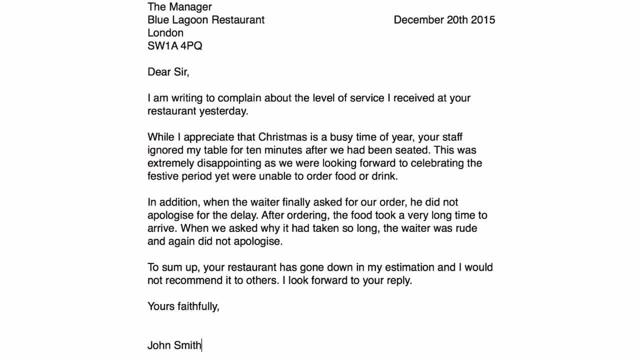 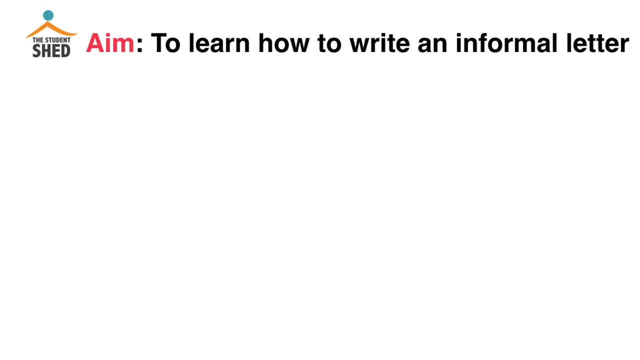 you can see that's a well-structured, formal letter that has all the right elements there. OK, so let's move on a little bit to look at informal letters, which is slightly easier than formal letters. They do, of course, have a different tone to a formal letter. First, 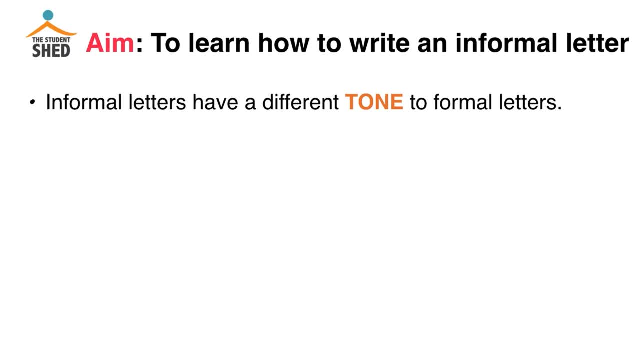 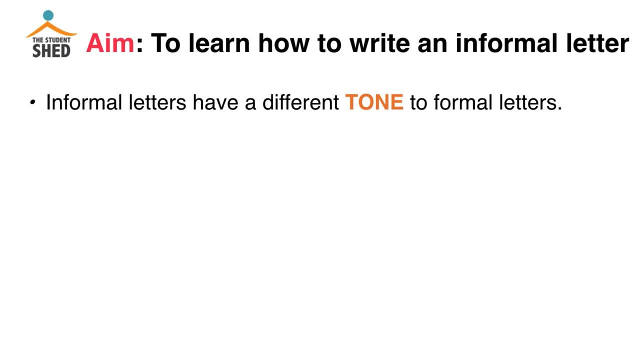 can start with much more informal terms, such as hi or hey, at the beginning of an informal letter. Your language, of course, can be much more chatty in style, because you're likely to know the person that you are writing to And the sign off is also informal. You can. 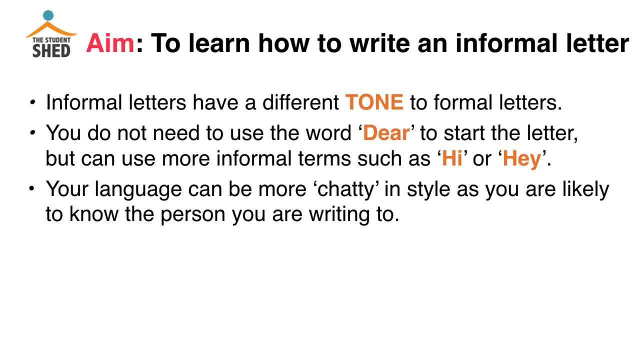 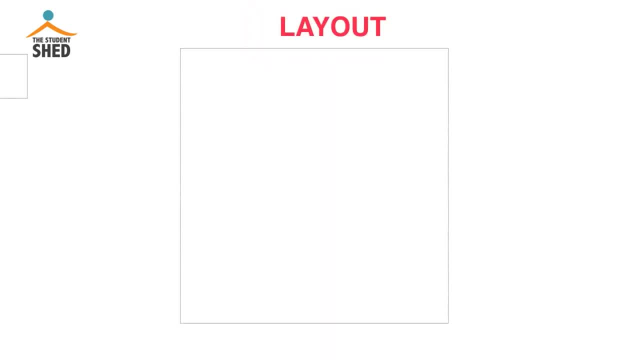 use lots of love or see you soon or any other appropriate informal sign off, rather than yours faithfully or yours sincerely. Now, the layout for an informal letter is always: the letter is not dissimilar to a formal letter, but the one big difference you'll notice is: 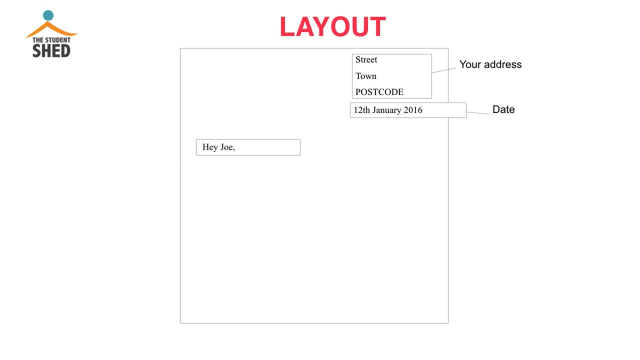 that you don't include the name of the person on the left side of the page. You just put your own address and your own postcode and the date on the right hand side, followed by the salutation there, which in this case is Hey Joe. Then you would have a polite introduction. 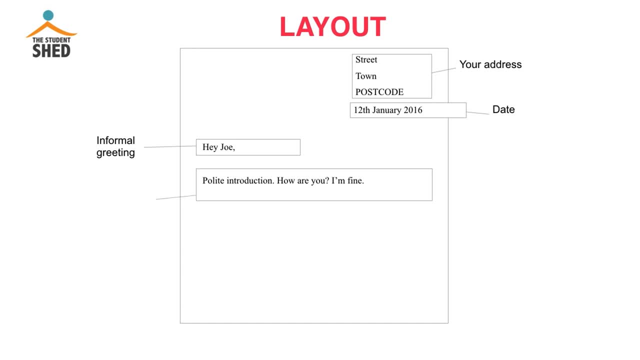 in using informal language. how are you? I'm fine, that kind of thing there in your opening paragraph, and then, of course, you'd move on to different topics depending on what you were talking about in the informal letter. When you conclude the letter, obviously you 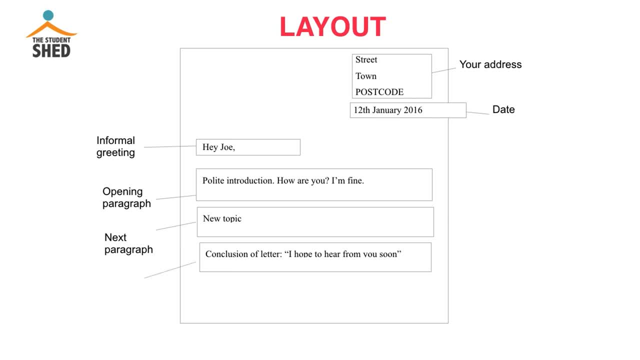 would talk about hoping to see them soon or hear from them soon, because they're likely to be a friend of yours. Then, as we said, the sign off can be informal, in this case, lots of love. and then, obviously, you would just sign the letter at the bottom with your 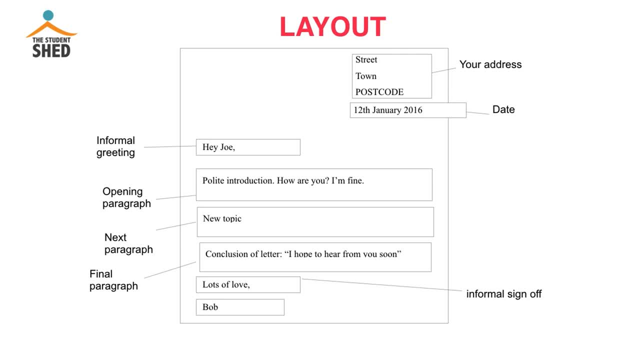 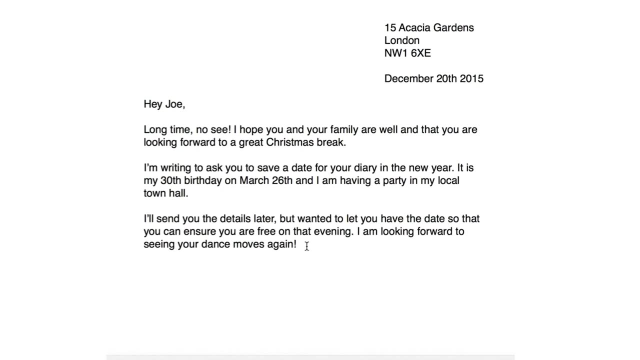 name with no need to print it as in a formal letter. So it's quite straightforward and easy. the layout of an informal letter. So here's an exemplar of an informal letter: the same address as previously, but this time no address. on the left, and rather than Dear Sir or Madam, it says Hey Joe, long time no. 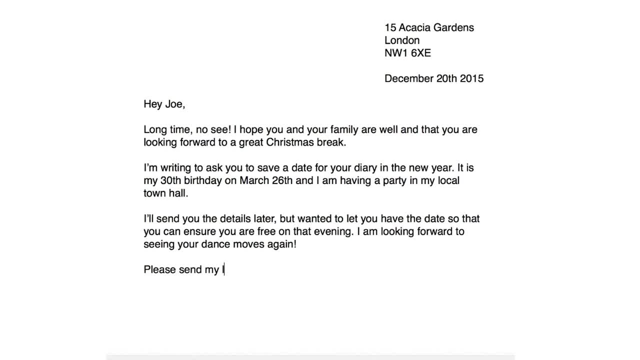 see nice and informal beginning there talking about his family, and then there's a date in the diary later on in the letter. there It finishes. Please send my love to your family and I look forward to seeing you all again in the new year, and this time rather than yours faithfully or yours sincerely, it's a straightforward. 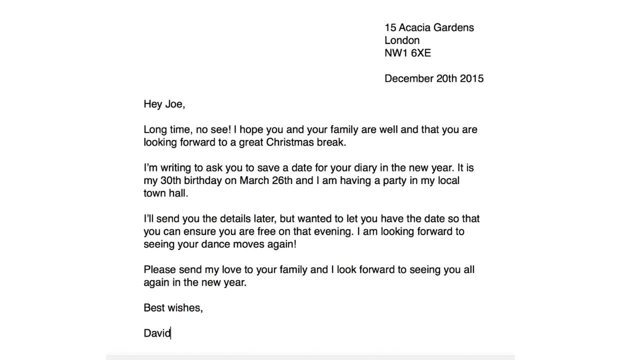 best wishes and David, there no need to write the name at the end of the, no need to print the name at the end of the letter for an informal letter. So there you go. there's an example of a quite straightforward informal letter for you to. 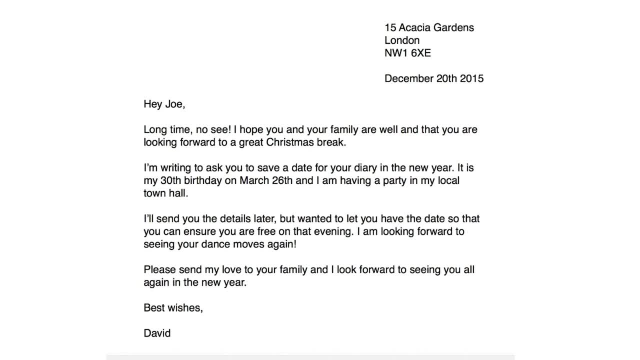 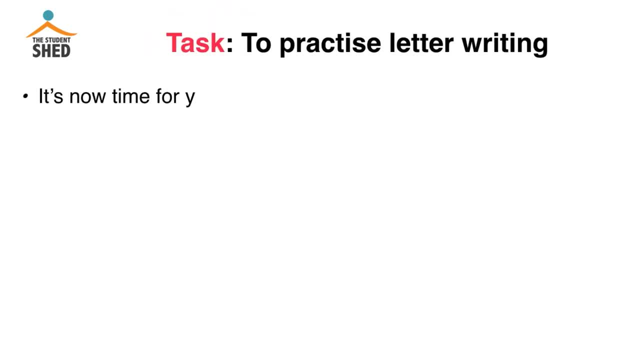 look at. You can pause here and read that through again if you would like to. Okay, so it's now done. So it's now time for you to practice letter writing yourself. So what we would like to do is to write two letters. a formal letter to a restaurant complaining 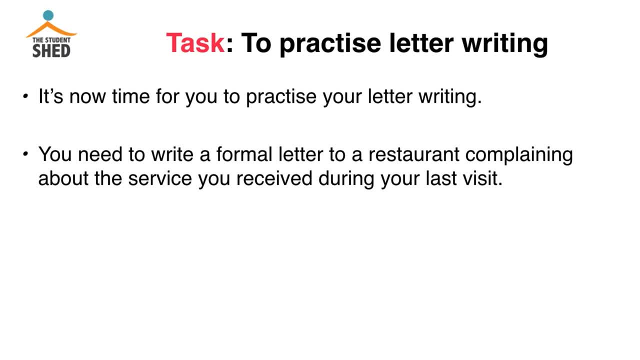 about the service you received during your last visit. So, in other words, very similar to the letter that we looked at earlier, but try to write one in your own words and change the scenarios slightly. and also an informal letter to a friend, like this to be about the same experience, where you recall the bad service in the restaurant. 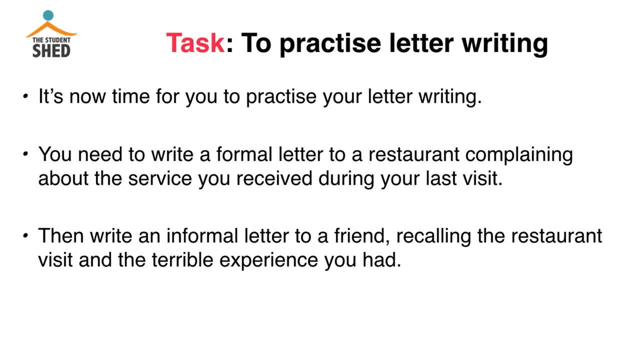 but you're writing a much more informal letter, much more informal letter to a friend, telling them what happened to you the previous evening. it's important that you remember to think about layout, to structure and tone and get that appropriate for each of the two different letters. okay, well, that is the end of today's lesson. please feel free. 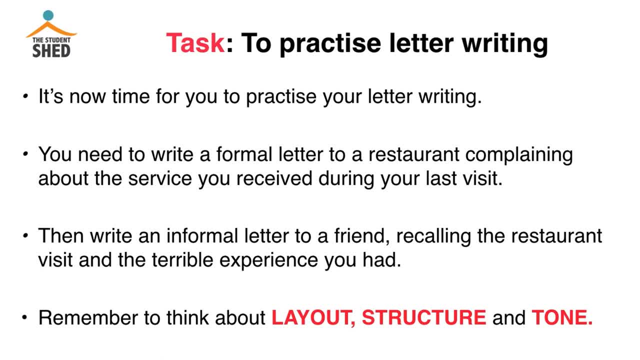 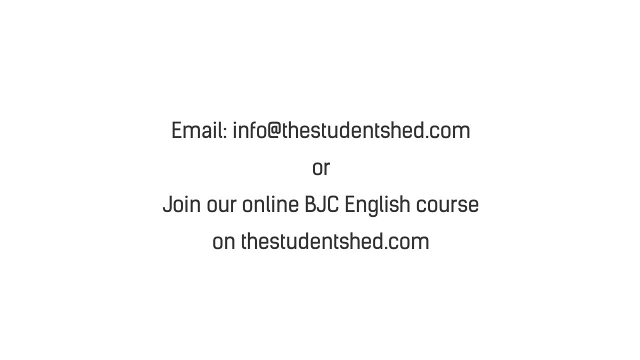 to rewind this presentation and carefully go through each of the bullet points again before you embark on your letter writing task, which should take you at least 30 minutes to complete. for more help, you can email info at the studentshedcom. goodbye.